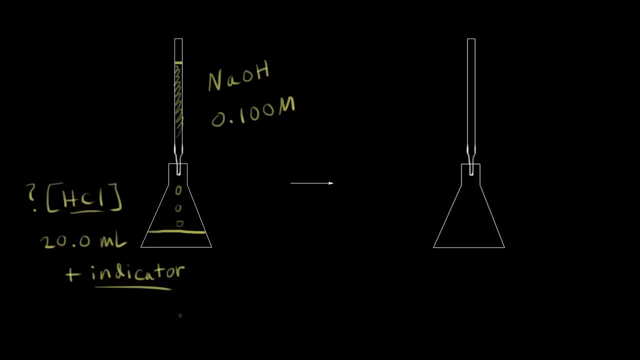 And the acid in the base will react right. So we get an acid-base neutralization reaction: HCl plus NaOH, right? If we think about the products, this would be OH minus, This would be H plus. H plus and OH minus give us H2O. 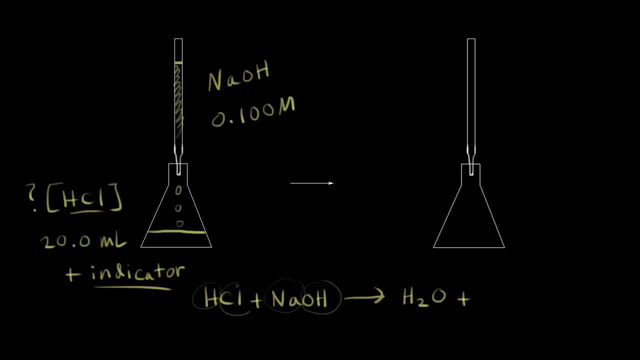 And our other products. we would have Na plus and Cl minus, which give us NaCl or sodium chloride. So let's say we add a certain volume of base, right? So now this would be higher And we see our solution turn light: pink, right. 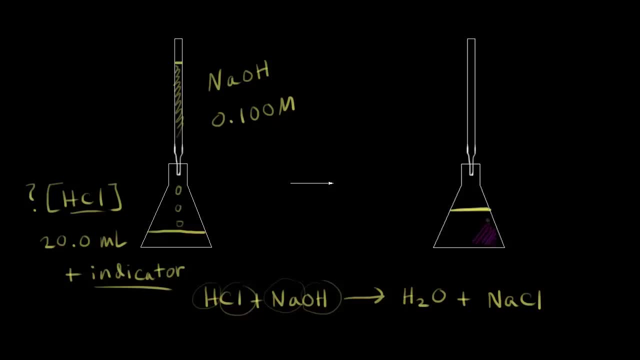 So let's say we see our solution turn light pink and it stays light pink. That means that all of the acid has been neutralized by the base And we have a tiny, a tiny amount of excess base present And that's causing the acid-base indicator to remain pink. 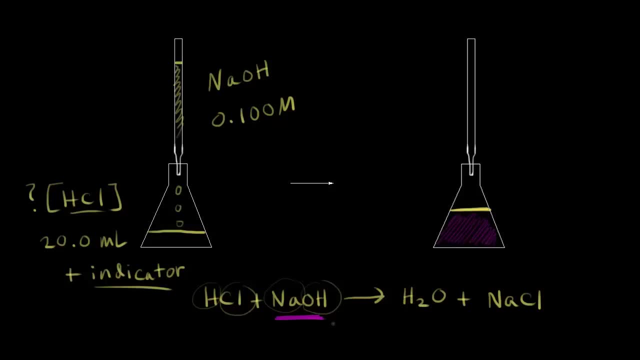 So a tiny excess of base means we've neutralized all of the acid present. And where the indicator changes color, this is called the end point of a titration. All right, So when our solution changes color, that's the end point of our titration. 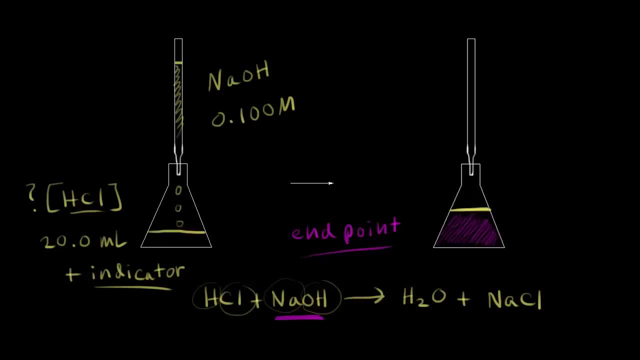 And here we stop and we check and see the volume of base that we used in our titration. So if we started right here, if we started with that much base, let's say we ended down here, So we still have a little bit of base left. 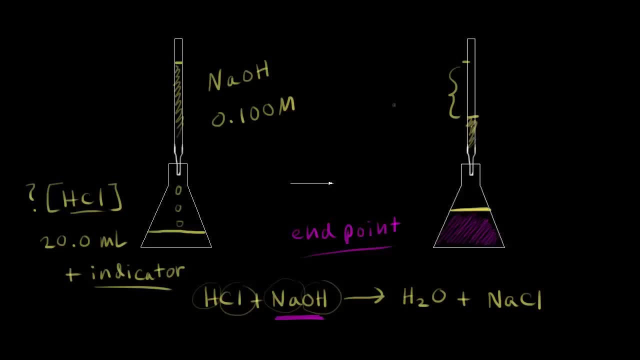 And this would be the volume of base that we used in the titration. So we have a change in volume here And let's say that it's 48.6 milliliters. So it took 48.6 milliliters of our base. 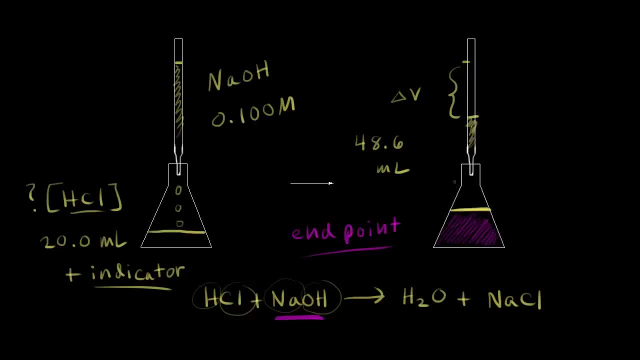 to completely neutralize the acid that we had present, And so we can now calculate the concentration of the HCl. All right, So let's go ahead and do that And let's start with the concentration of sodium hydroxide, All right. 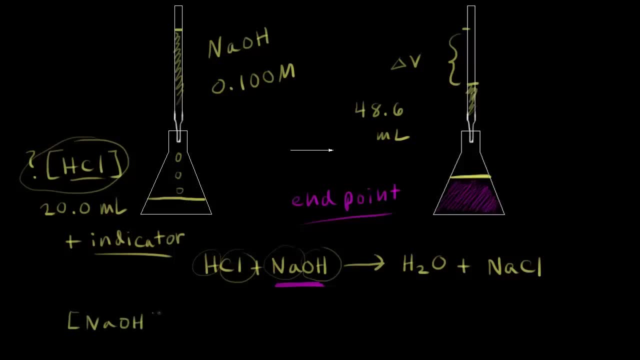 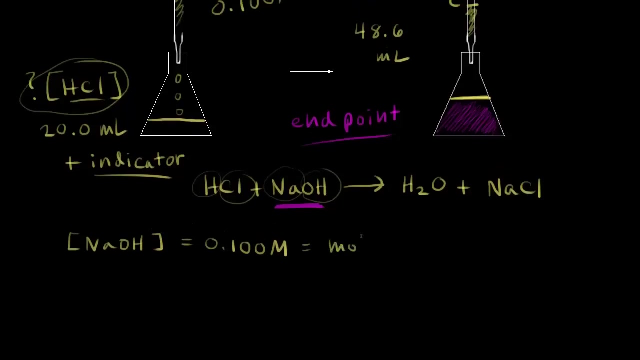 We know that we started with 0.100 molar solution of sodium hydroxide, So 0.100 molar And molarity. molarity is equal to moles over liters. All right, So this is equal to moles over liters. 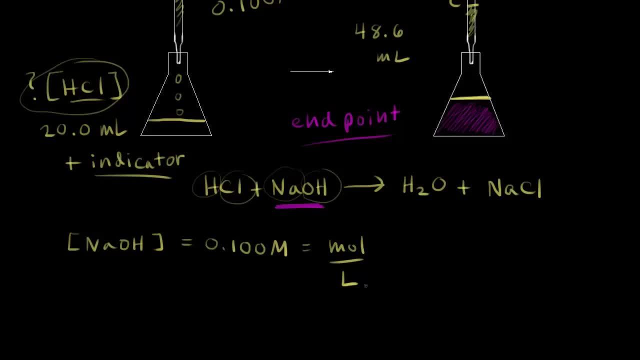 And our goal is to figure out how many moles of base that we used to neutralize the acid that was present. All right, So we can take our volume here, 48.6 milliliters, and we can convert that into liters. 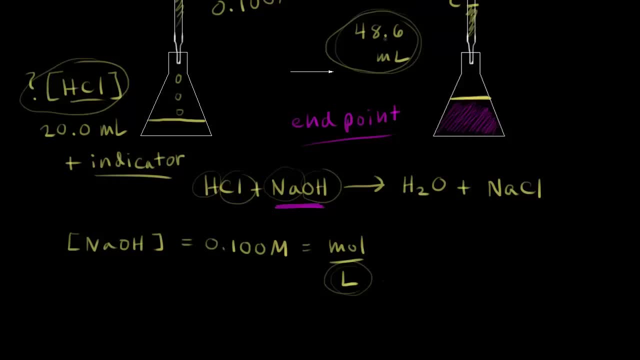 All right. So just move your decimal place three places to the left. So one, two, three, So that's 0.0486 liters. So this is equal to moles over 0.0486 liters, And so let's get some more space. 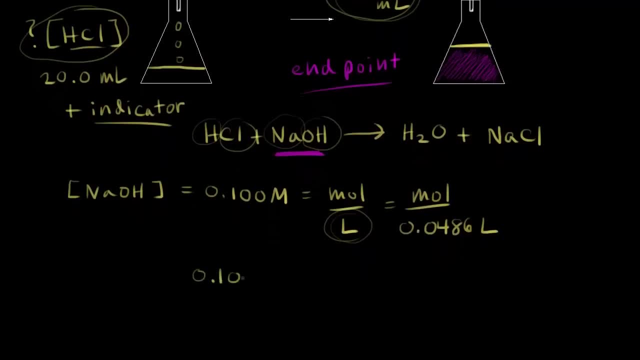 All right, Let me just rewrite this really quickly: 0.100 is equal to x over 0.0486.. So we're just solving for x, And x represents the moles of sodium hydroxide that were necessary to neutralize. 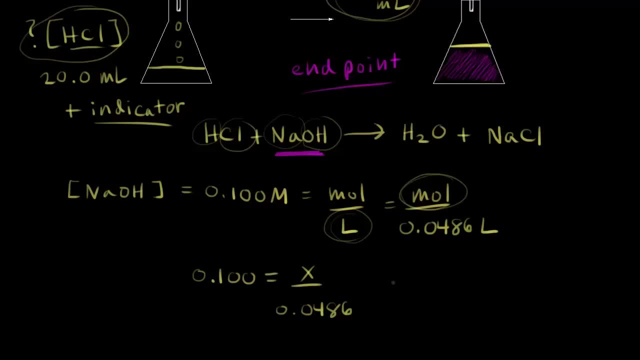 the acid that we had present. All right. So when you solve for x, you get 0.00486 moles of sodium hydroxide used in our titration. Next you look at the balanced equation. for what happened? All right. 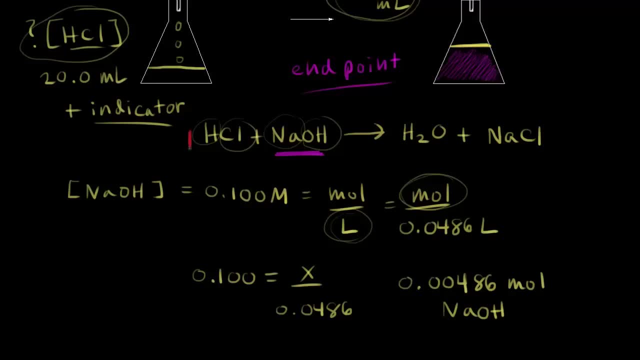 So if I look at my balanced equation, all right, there's a one here, right, and there's a one here. So we have a one-to-one mole ratio And the equivalent of that. the equivalence point is where? just enough of your standard solution. 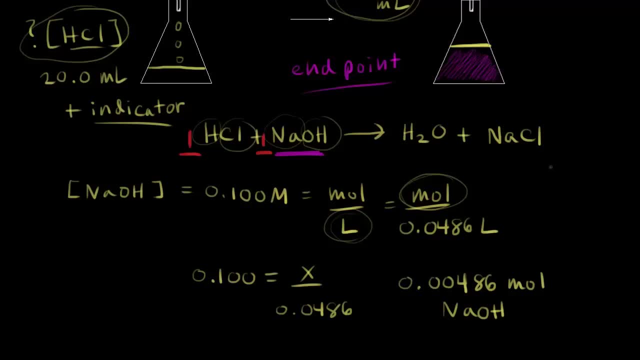 has been added, to completely react with the solution that's being titrated And at the equivalence point all of the acid has been neutralized, All right, So it's completely reacted. And since we have a one-to-one mole ratio- right, if I use this many moles of sodium hydroxide- 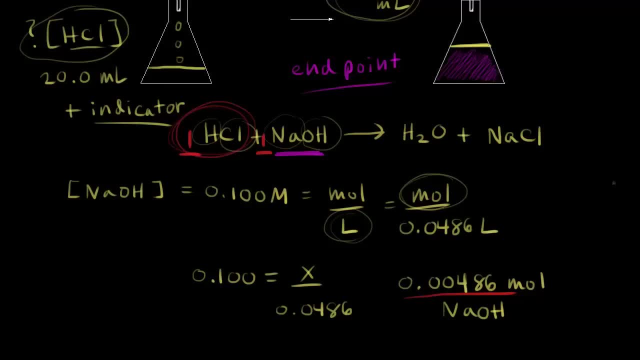 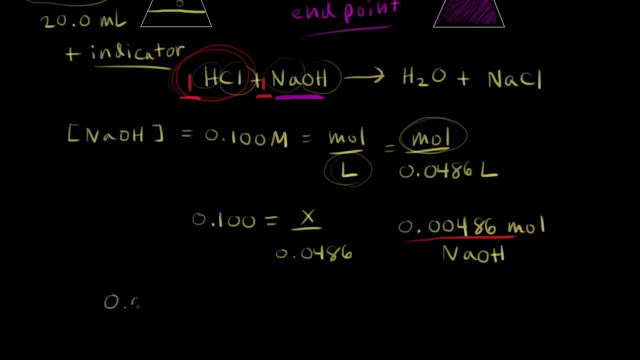 that must be how many moles of HCl that we had present in our original solution. So therefore I can go ahead and write that I must have had 0.00486 moles of HCl present in the flask before we started our titration, right? 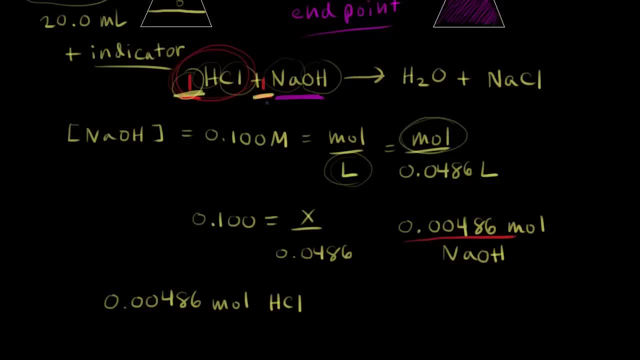 And I knew that because of the one-to-one mole ratio. All right, remember, our goal was to find the concentration of HCl right. the original concentration And concentration molarity is equal to moles over liters, So now I know how many moles of HCl I had. 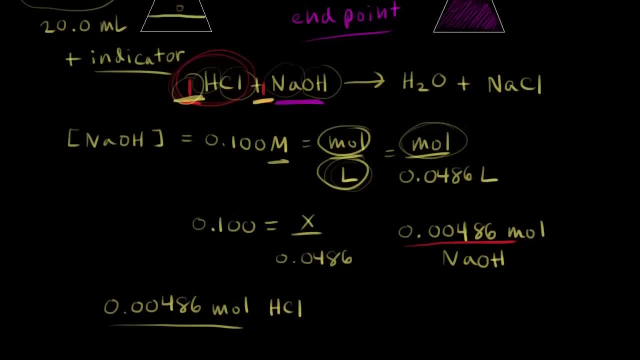 and my original volume of HCl was 20 milliliters, right. So right up here we had 20 milliliters. So I need to convert that into liters. So I move my decimal place one, two, three, So I get 0.02 liters. 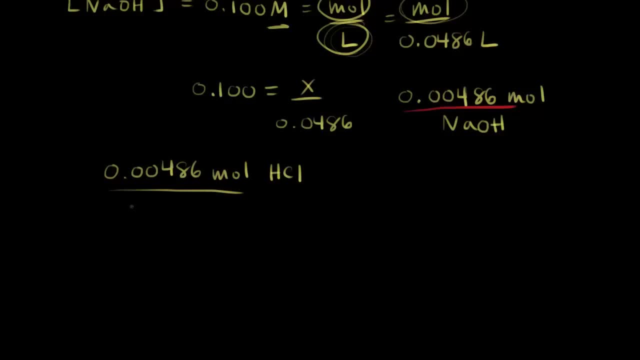 So now our final step here, to calculate the concentration of HCl. all right, so the concentration of HCl is equal to how many moles of HCl we have, which is 0.00486.. All right, So that's moles over liters of solution. 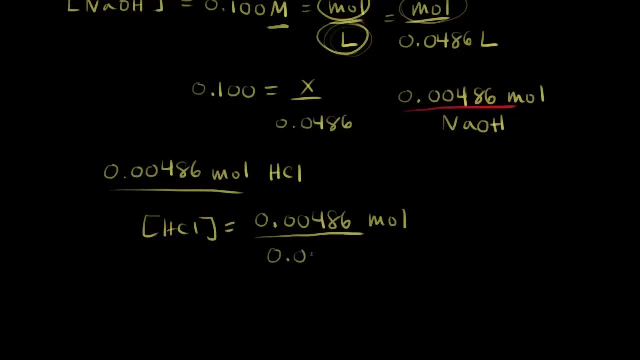 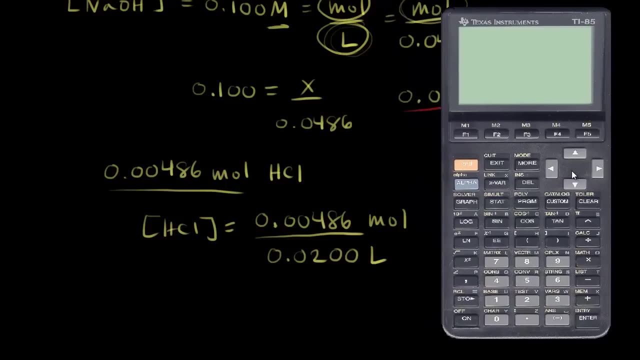 And we had 20 milliliters, which is equal to 0.0200 liters. All right, so now we can take out our calculator and do this calculation to find the concentration of HCl that we started with 0.00486,. all right. 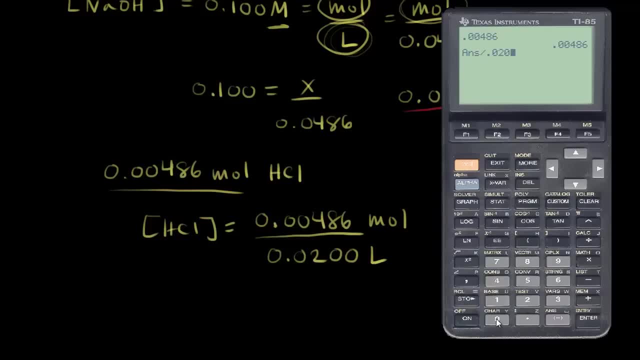 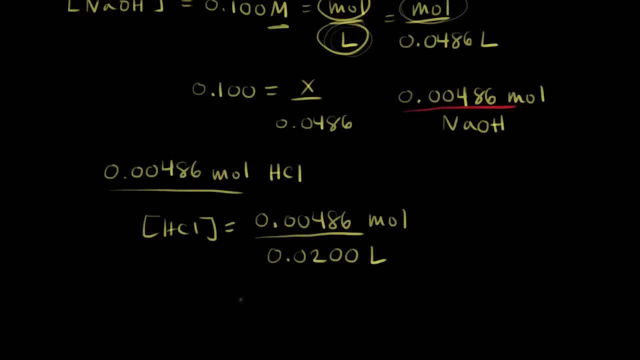 And we're gonna divide that by 0.0200.. And we get 0.243 for our answer. So the concentration of HCl, all right, is equal to 0.243 molar. So we've solved. we've solved for the original concentration of HCl. 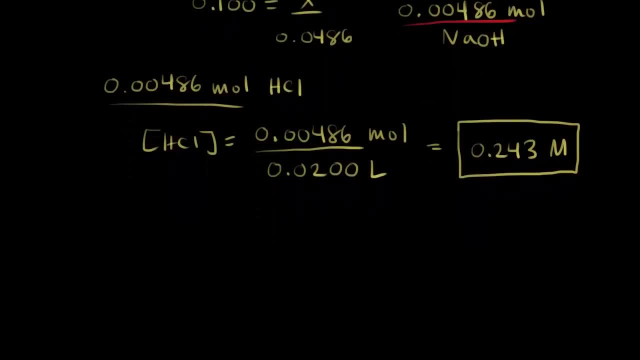 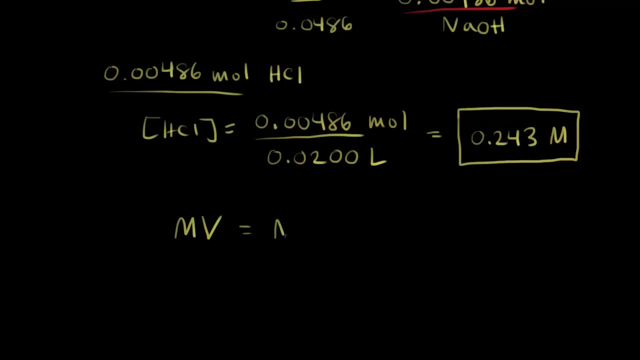 There's a shortcut way to do this problem. all right, And the shortcut way would be to do the molarity times. the volume of the acid is equal to the molarity times the volume of the base used, So MV is equal to MV. 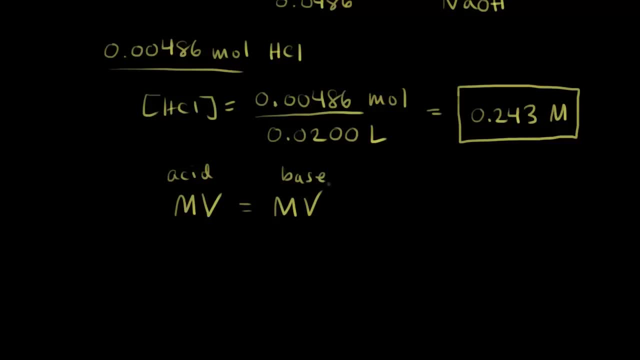 So let's say we have the acid over here on the left and the base over here on the right. So the molarity of the acid is what we're trying to find. So I'll just make that X The volume of the acid that we started with. 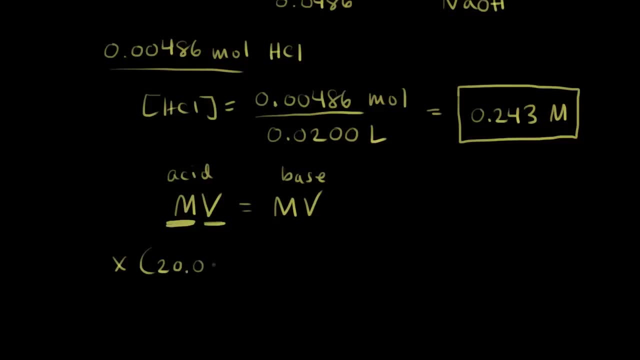 you can just leave this in milliliters if you want. 20.0 milliliters is how much of the acid we started with And for the base, we knew the concentration of the base that we used in our titration right. 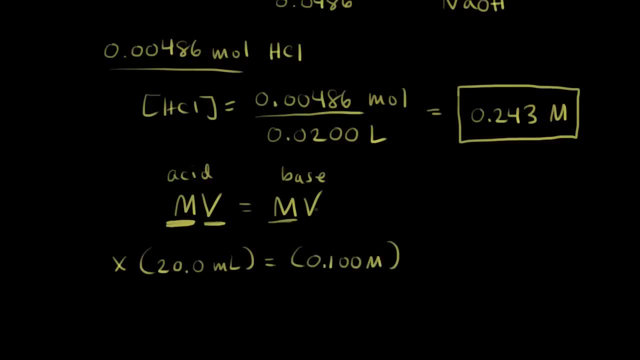 It was 0.100 molar And we also knew the volume of base that we used to completely neutralize the acid. We used 48.6 milliliters And notice how the mLs would cancel out here. all right,